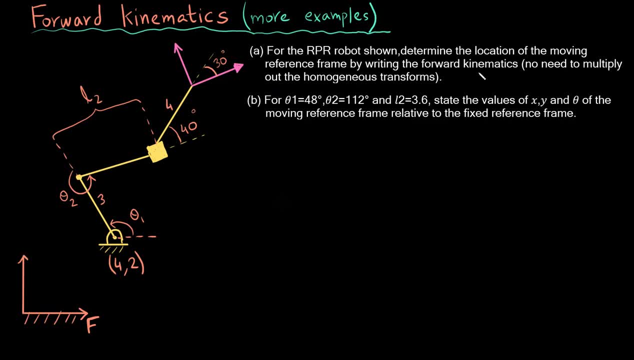 So it just asks us to write out the homogeneous transforms as h1, h2, h3 and so forth, and there is no need to multiply them out. And the second part says that for theta1 as 48 degrees, theta2 as 112 degrees and L2 as 3.6,, state the values of x, y and theta of the. 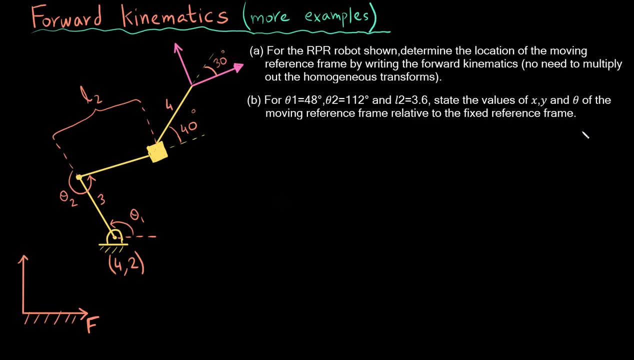 moving reference frame relative to the fixed reference frame. So in part b all we need to do is, from the homogeneous transform that we obtain in part a, we are going to input the specific values of theta1,, theta2 and L2 and get the final homogeneous transform and from that we can extract the x- y values, which 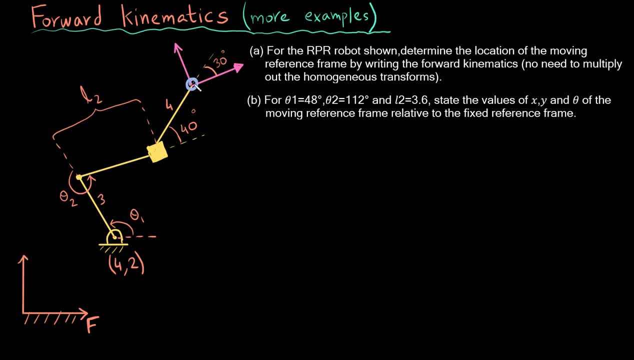 are the values of the final moving frame in the fixed frame, and also from that we can get the theta, which is the orientation of this moving frame in the fixed frame. So kind of this. Before we move on to part a, let me just draw out the moving frames at each of the joints. 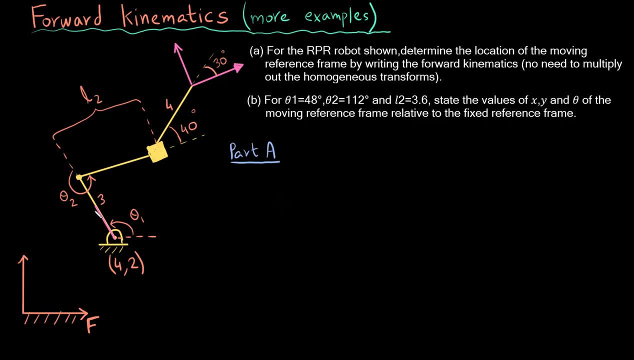 So the first moving frame is going to be here, with the x-axis pointing here and the y-axis pointing here. The second moving frame is going to be here, with the x-axis pointing along this link, The y-axis perpendicular to it. The third is going to be here, The x-axis pointing along this link. 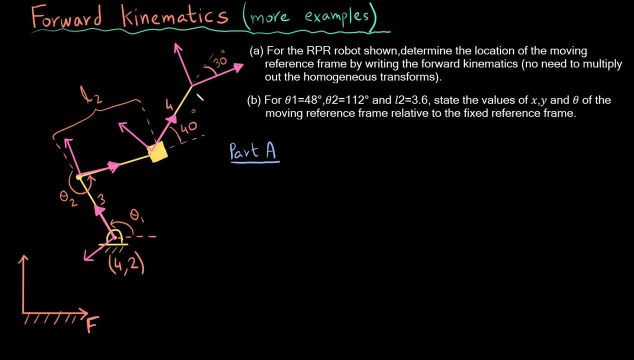 And the y-axis here. And for the fourth, we have already been given this reference frame. So I call this one m1.. Moving frame 1, this one m2, this one m3 and the final one is m4.. So what we need to do is, in part a, we need to go from 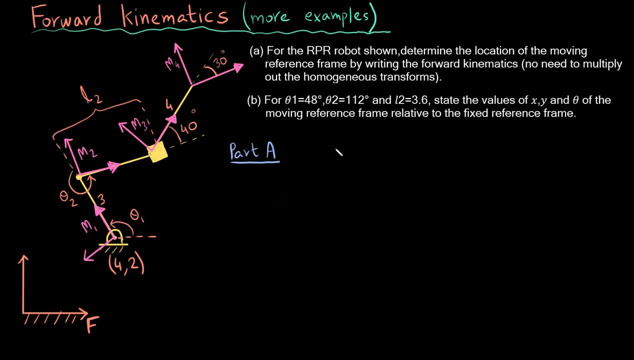 The fixed frame to the m1 frame, m1 frame to m2 frame to m3 frame and finally to m4 frame. So I am going to make use of A number of homogeneous transforms. I'm going to use H1, which takes this from to this and then this from here to here. So 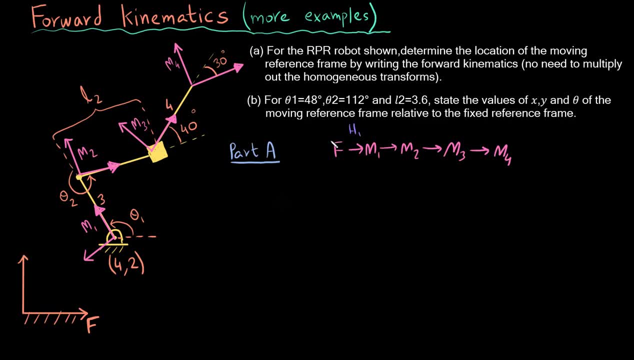 I am going to use. I am going to use a number of homogeneous transforms. I'm going to use H1, which takes this from. to this, I'm going to use a number of homogeneous transforms. these two. then i'm going to make use of h2, which takes m1 to m2, and similarly h3 and h4. 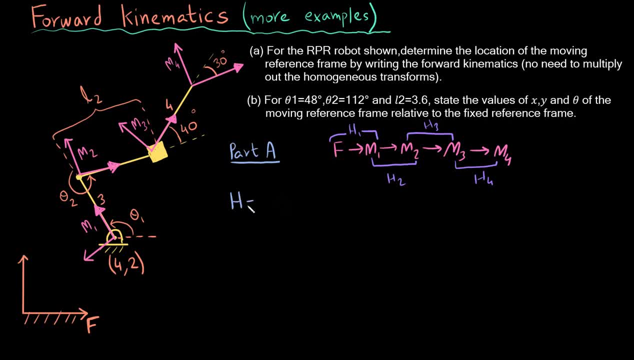 so the homogeneous transform that i want is h1 times h2 times h3 and h4, where the h1 is going to take the fixed frame to this point, the h2 is going to take m1 frame to m2 and the h3 is going to take this to this point, right here, and the h4 is going to take this to. 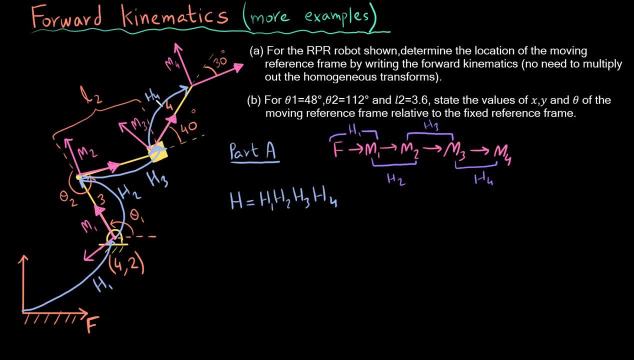 here. i hope the diagram isn't too messy to understand, so writing it out. i can write h1 as a rotation matrix with an angle of theta1 and then there are two zeros. i can write zeros as zero vector transpose, then the displacement is four and two and one. similarly, the h2 is going to be the moving frame, m2 with respect to m1, so the rotation. 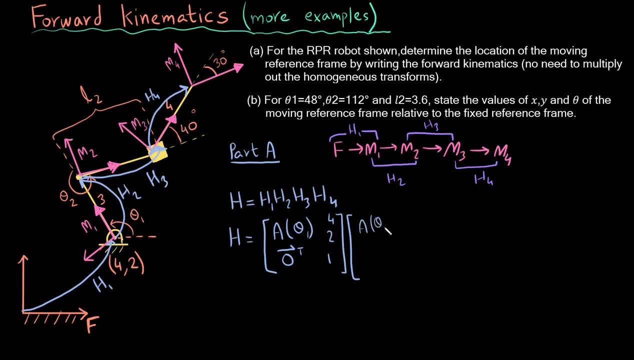 is going to be theta, two, zero, transpose, and three and zero and one, and h3 is going to be m3 with respect to m2. so here the rotation is going to be just 40 degrees: zero, transpose. the displacement here is going to be a, 2 and x and 0 and y and 1 and for the final frame, h4. 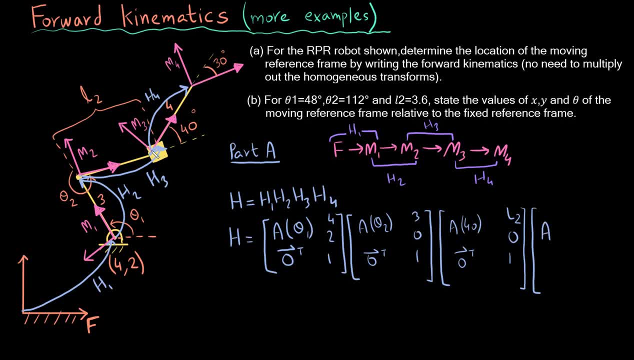 now for the final frame, h4, my, when i displace m3 to this point, the x-axis is along this line, so i can take it all the way here, which is going to be 330 degrees, or, since i know counterclockwise is positive, so clockwise must be negative. 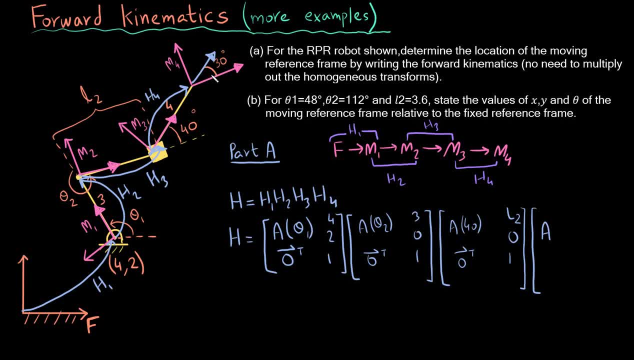 so i can use this, which is minus 30 degrees, since i am going in the clockwise direction, so i can write this as minus 30. this is 0, transpose: uh, the displacement is four units, and x, zero and y and y, and this is the answer to part one, since they have also 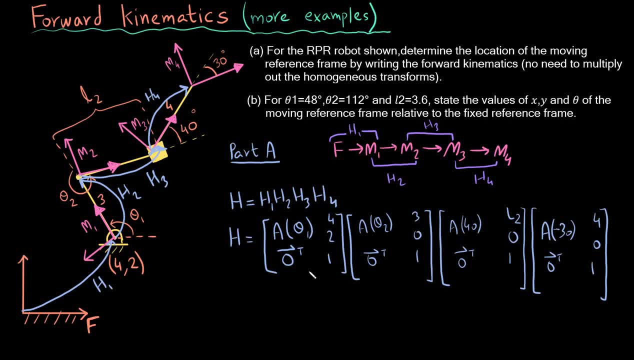 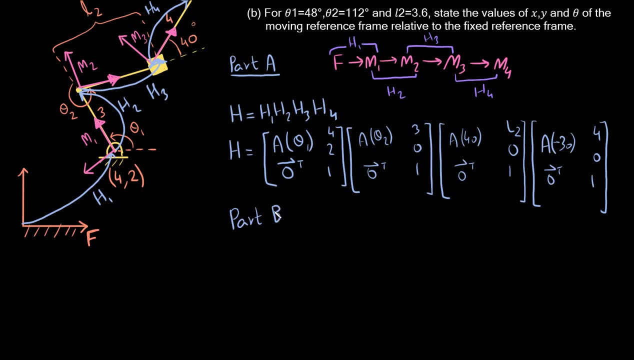 this, that there is no need to multiply. so you would multiply it out, and this is the answer that we get for part one. so part one is done now, moving to part two. so in part two, all we need to do is we need to just import the values that they have. 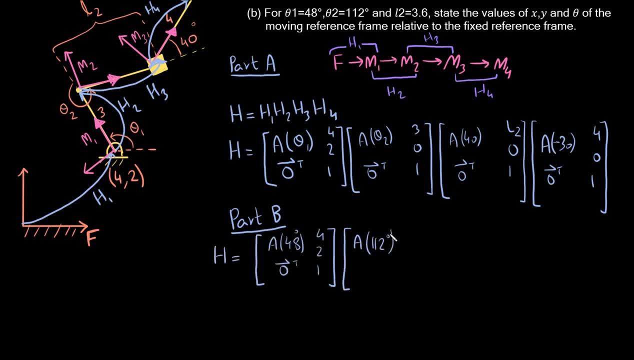 provided us. so I hope you do remember that this a that I am writing everywhere is the rotation matrix, which is of the form of cosine of Theta, sine of theta, minus sine of theta and cosine of theta. so this is my a matrix, so if I am writing a of theta, so 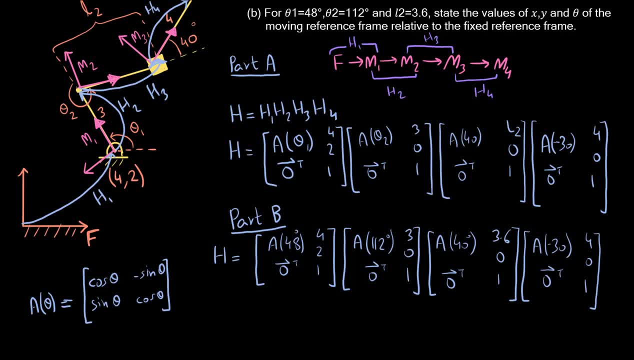 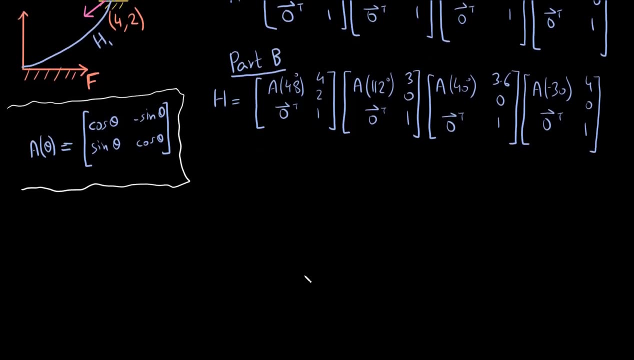 this is what I mean by a of theta. I just want you to put it out, just in case you forgot. so this is what I mean by theton matrix. now, once I multiply it out, what I get is: so this is the homogeneous transform. transform that I get and this edge takes. 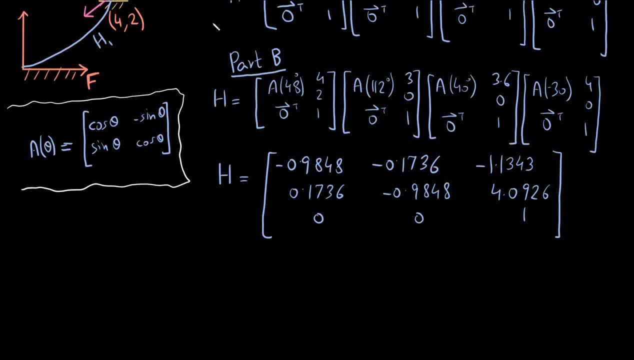 the fixed frame and takes it directly to the final moving frame, m3. from this I can directly reduce that these two numbers are the X and Y coordinates of the final moving frame. so this is my X, this is my Y. so if I go up in the 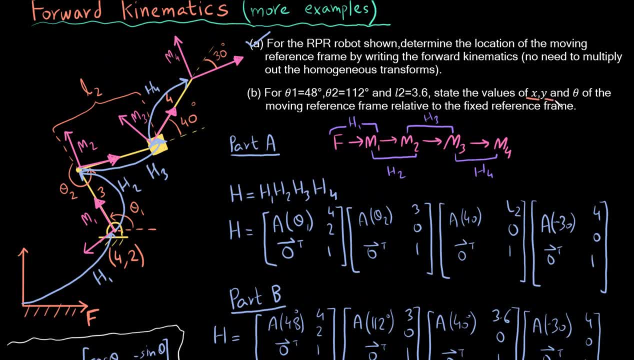 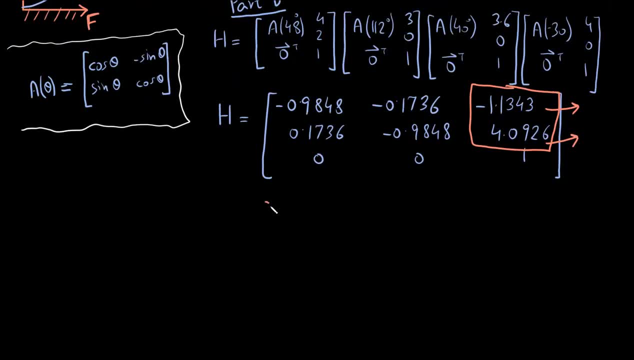 question. it asked me to find out the X, Y and theta. so directly from looking at this final transformation matrix that I get, I can say that my X is minus one point one, three, four, three, and X is minus one point one, three, four, three, and my Y is four point zero, nine, two, six. this is very easy. now I need to find out. 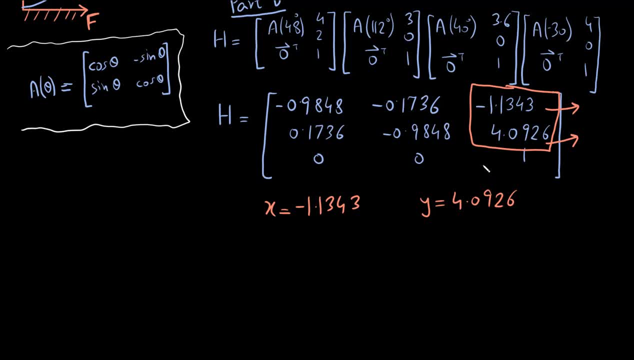 the theta, which is orientation of the final moving frame with respect to the fixed frame. so I know that this part right here, the first two by two matrix, is just a rotation matrix and we know that the rotation matrix always takes this form. so by comparing the two we can see that this 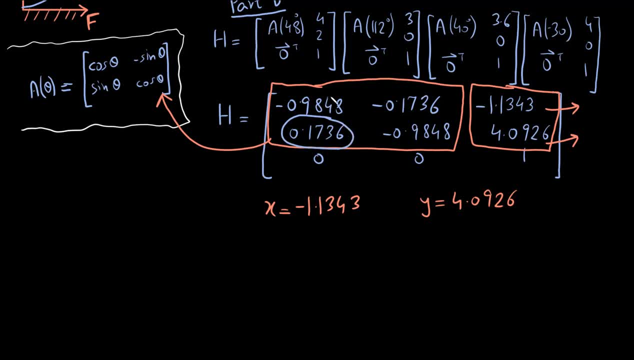 term right here is going to be sine of theta. this term right here is going to be cosine of theta. so I can write that the sine of theta or cosine of theta would be equal to. the sine is point one, seven, three, six. cosine is minus point nine, eight. 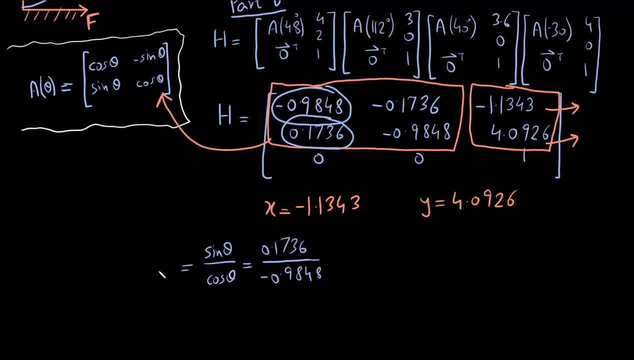 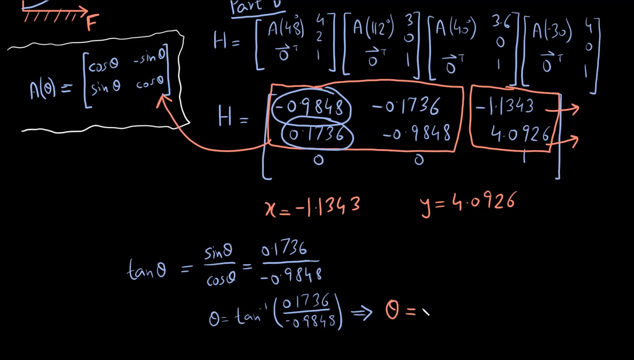 four, eight, and sine over cosine is 10 of theta. so if I just solve it out, I get theta to be equal to the 10 inverse of this, and this gives me the theta as equal to 170 degrees. so these three are my answers for part B. this is my X coordinate, this is my Y coordinate of the moving frame and 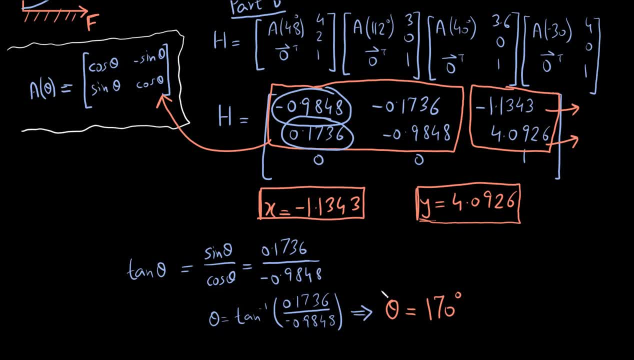 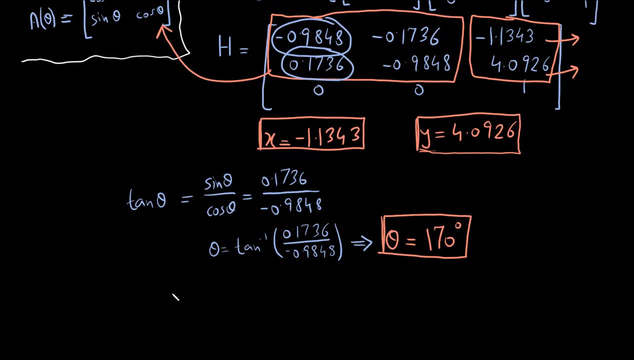 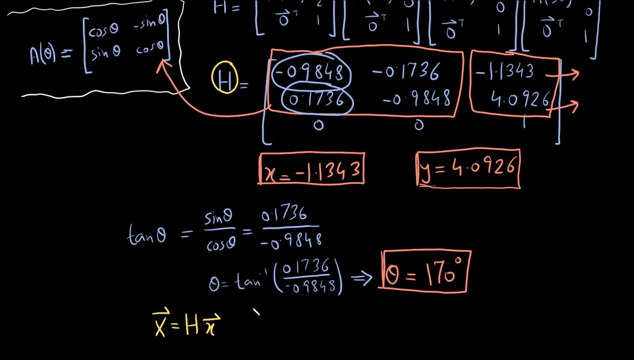 this is my theta. now I could have, of course, done it another way. I could have used this equation right here, which is: big X equals H times x, with the H being this H, right here. and if I wanted to find out the coordinates of the moving frame.